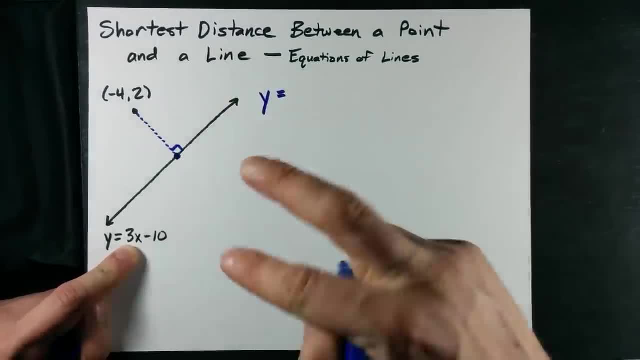 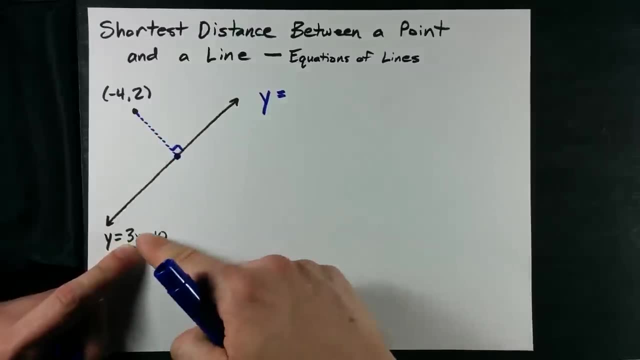 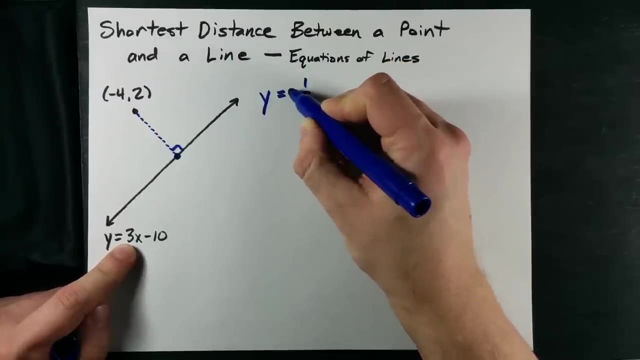 we now know the slope of this line segment because it has to be a negative reciprocal of this slope in order for it to be perpendicular. The negative reciprocal is what you get when you take this slope and you flip it and you make that number negative, or rather, you switch the sign: A positive slope becomes a negative. 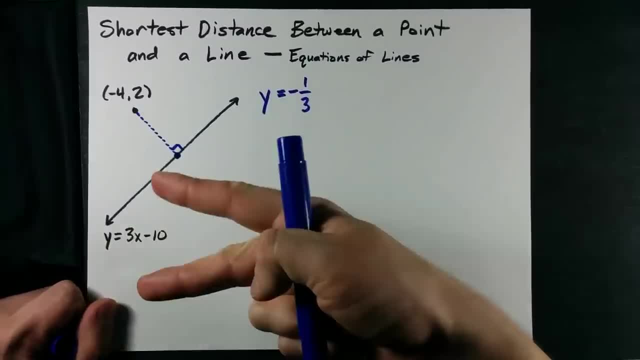 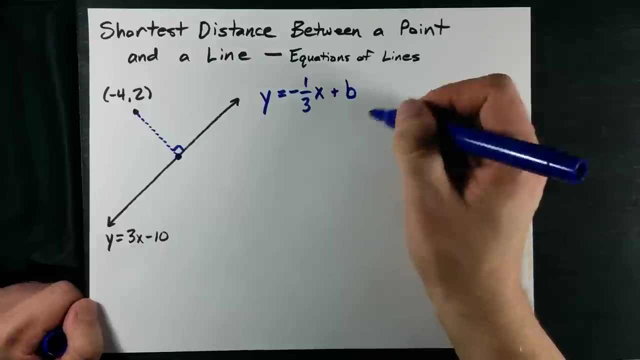 slope. So this fraction 3 over 1 becomes 1 over 3, and we change the sign. y equals mx plus b, as always. Now to solve for b, which you need if you want the equation of the line, you have to plug in. 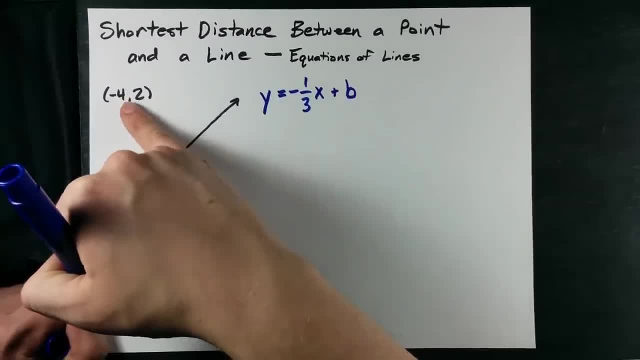 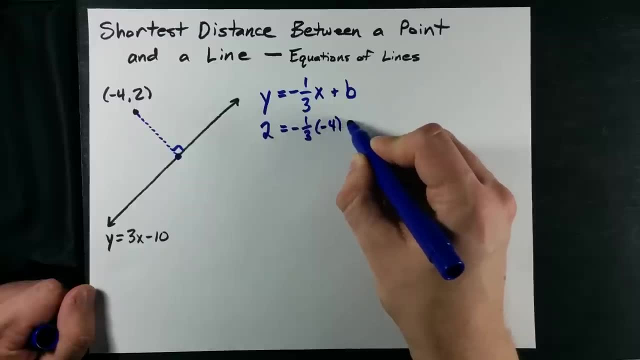 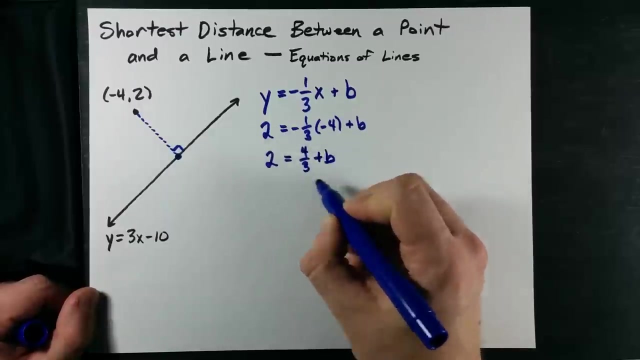 a point. The point that you know is on the line. that's where the coordinates you're given come in. That's negative 1 third of negative 4 plus b. Let's solve this. We've got 2 equals 4 thirds plus b. 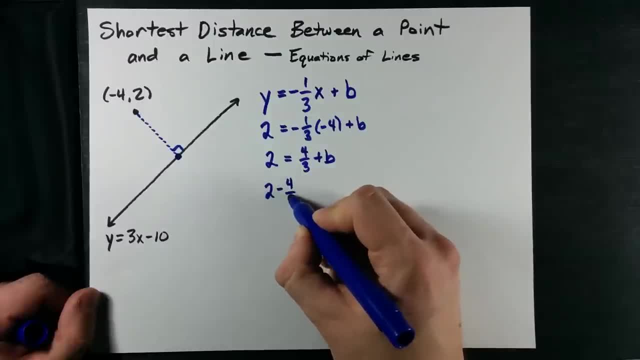 I'm going to move the 4 thirds to the other side. Oops, that's an equals And I don't know how you are with fractions. Worst comes to worst. you use your calculator. I guess I don't really care. 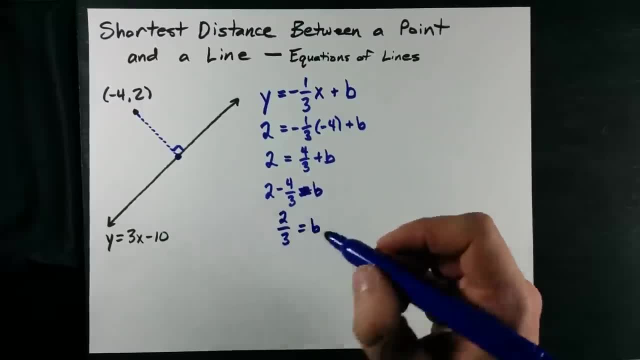 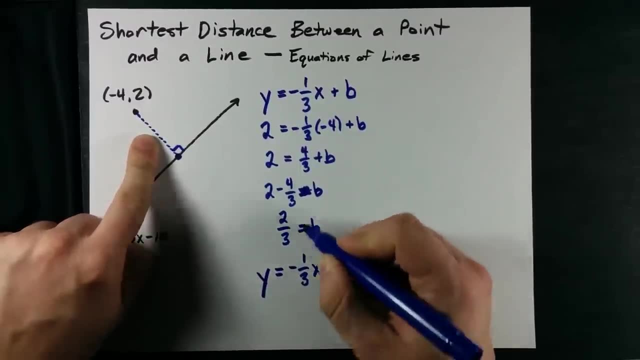 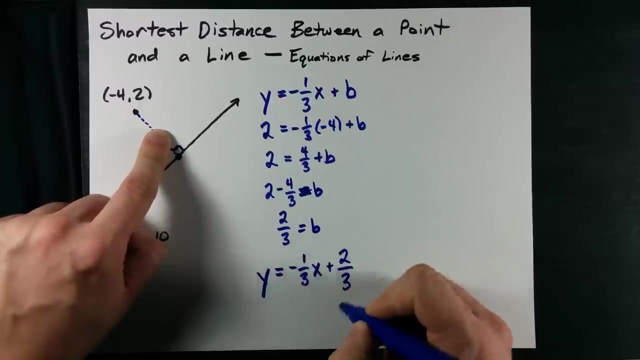 You're going to end up with. b is 2 thirds. Thus, the equation of the blue line segment is: y equals negative 1 third x. That's the slope from the beginning negative reciprocal of this one plus whatever b you solved for All. right Now in order to get the coordinates of this point. 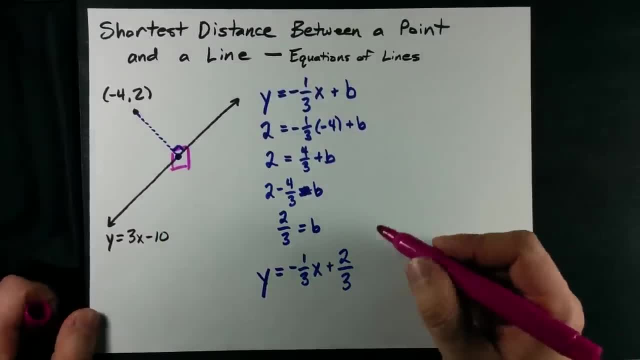 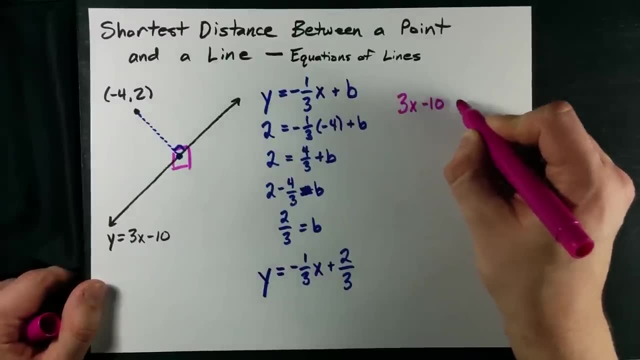 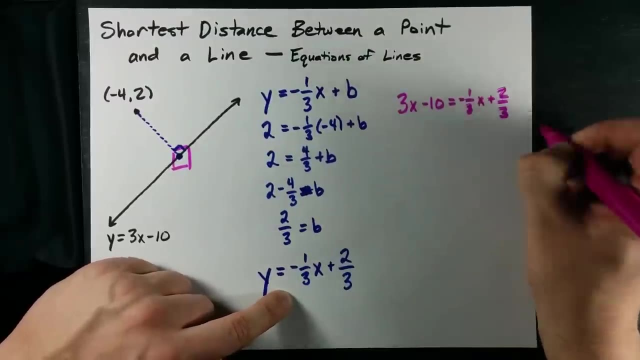 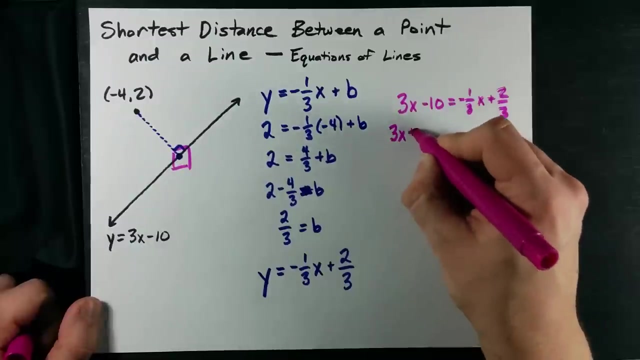 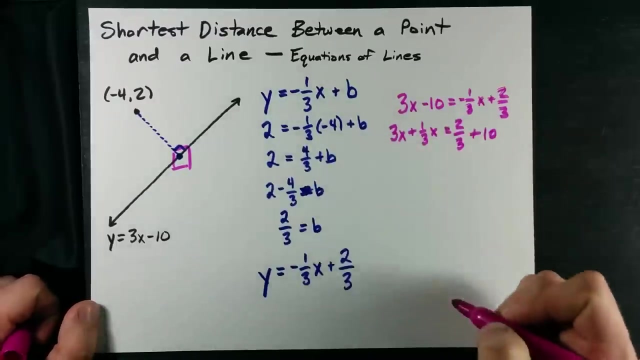 we need to find the point of intersection, Because both of these are in y equals. it's not perfect, But if I start to find the points, I'm going to get the to the last point of intersection. Alright, Let's try again. It's not perfect. I'm going to get y equals b as well. That's a point of intersection sign. I'm going to get y equals mx plus b form. I can just set them equal to each other. 3x minus 10 equals negative. 1 third x plus 2 thirds. I'm going to put all my x's on one side, all my numbers on the other. That's 3x plus 1 third x on the left and that's 2 thirds plus 10 on the right. That gives me. 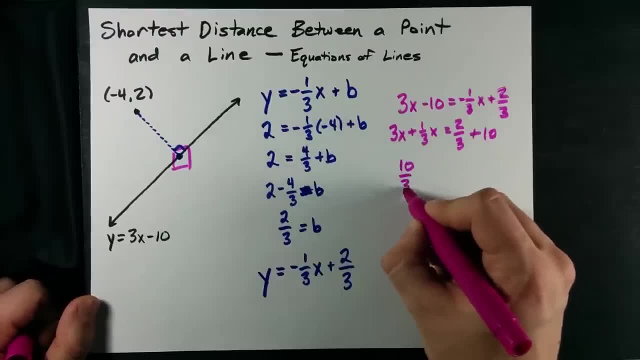 Now I'm going to do this. Now I'm going to do this. I'm going to do this. Now I'm going to do this. do my fraction work in my head here. That's 10 thirds of x here and this is 32 thirds here. 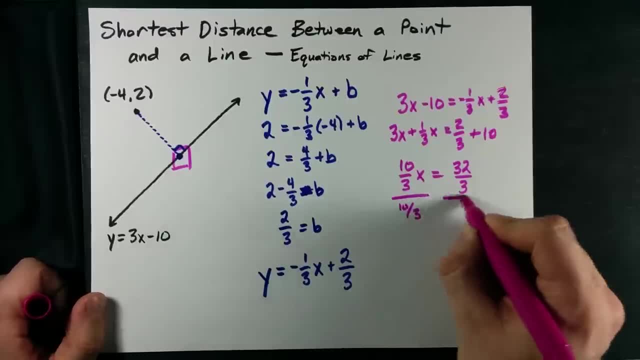 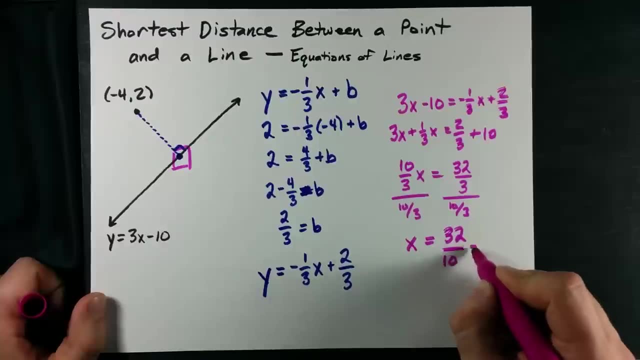 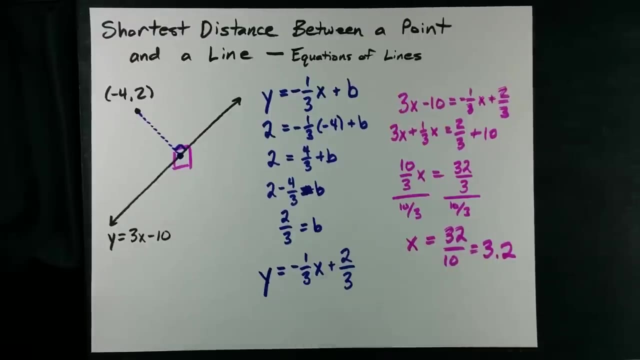 Then, in order to solve for x, I divide both sides by whatever is in front of x. When I do that, I get 3.2.. I did that on my calculator in case you're curious. Just kidding, But you can use your calculator, It's totally allowed. So the x coordinate of that point is 3.2. 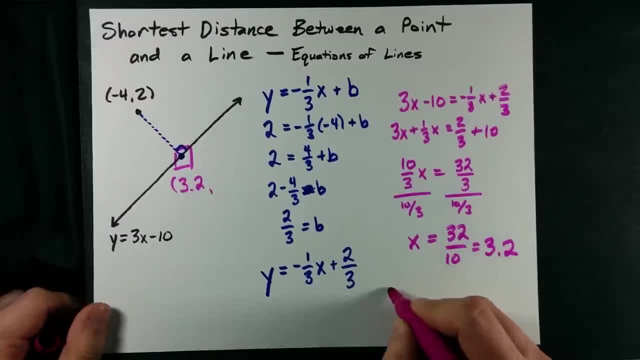 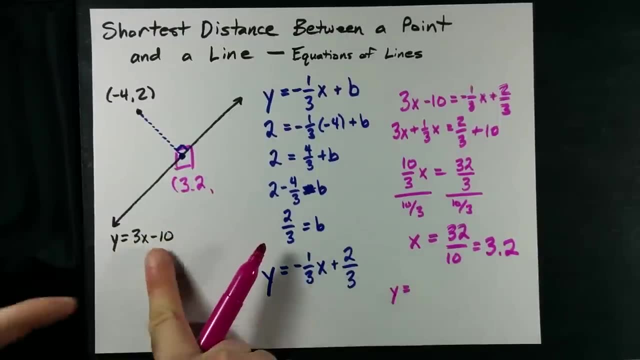 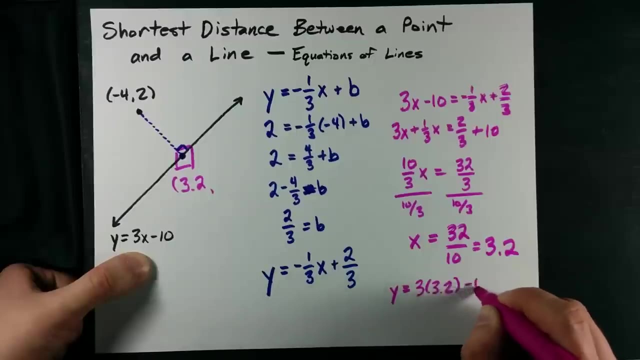 I wish I knew what the y coordinate was. Well, we can figure that out. You're allowed to plug that x value into either of these equations to get the y value. I'm going to plug it into the one that scares me the least. That's this first one. 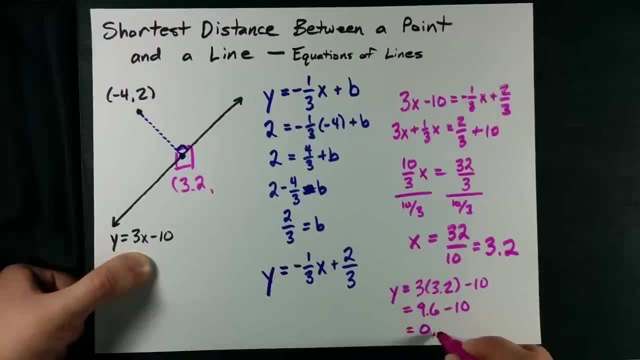 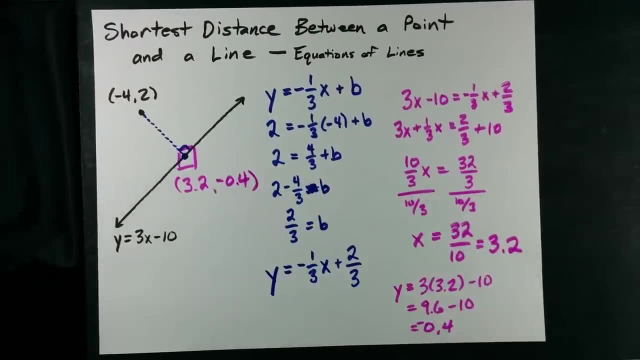 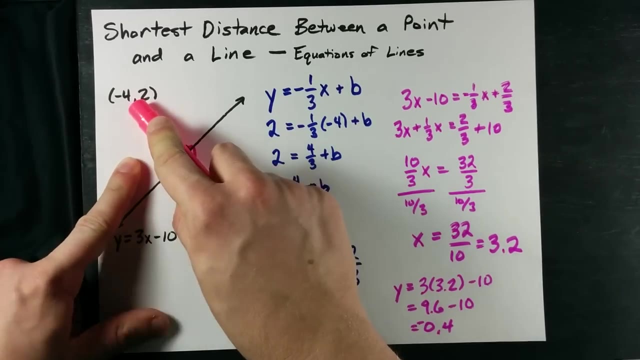 That's 9.7.. 6 minus 10, so it turns out to be negative 0.4.. Cool, Let me reiterate how we did that. I found the equation of the line perpendicular to this one that went through that point. 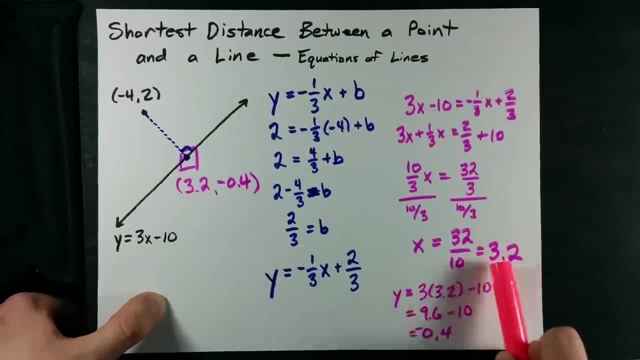 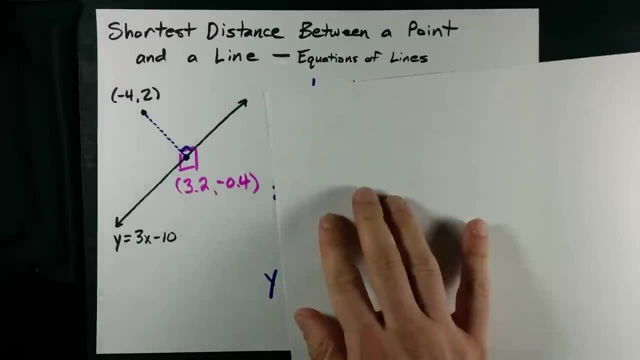 Then I set the two equations equal to each other to get the x and y where the two intersected. Now we're still not done, Because they actually asked for what the distance was between those two. I have to use the distance formula for that. 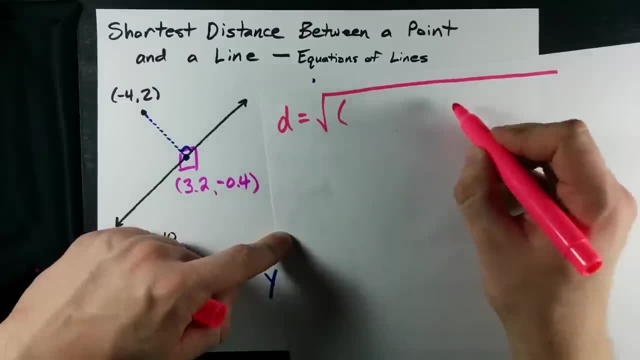 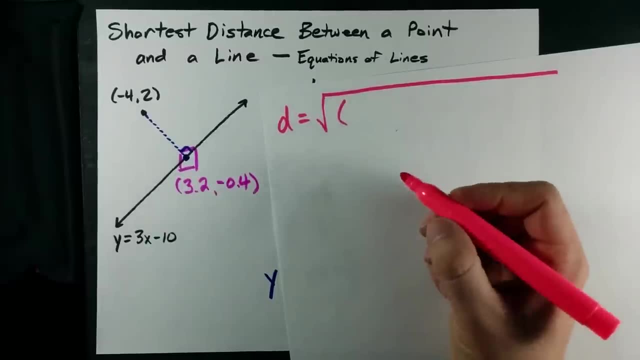 That's x2 minus x1 squared, plus y2 minus y1 squared. If you're in grade 10, it's probably going to be given to you. If you're beyond grade 11, you should have memorized it or used the Pythagorean theorem or whatever. 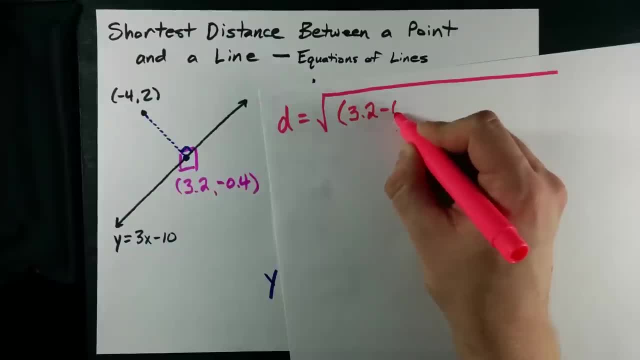 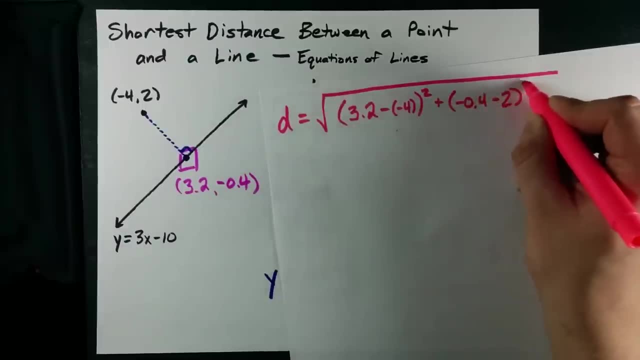 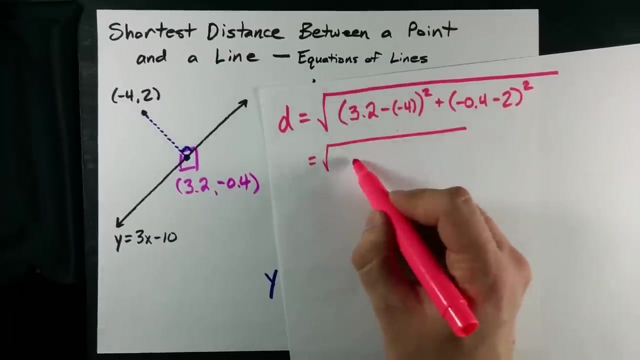 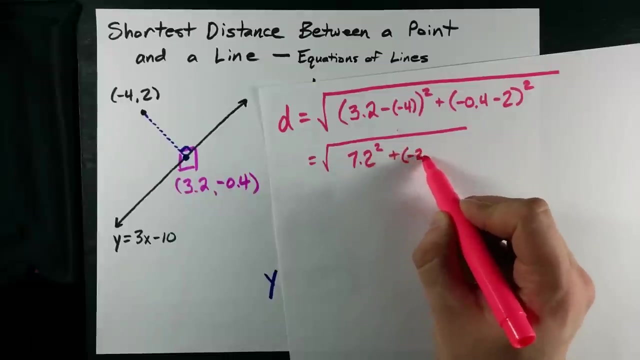 x2 minus x1.. All squared, y2 minus y1, all squared Added together and then square rooted. La la, la, this is just me doing work right Here. I get 7.2 squared plus negative 2.4. all squared: